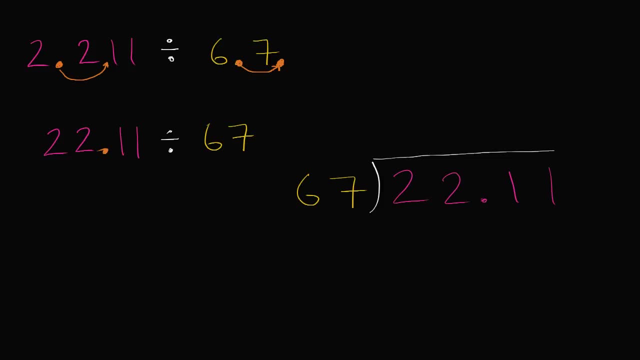 All right, let's do some long division now, And actually before we even do that, I like to keep track of my decimal. So my decimal is over here. I'm gonna write my decimal right over here in the answer And when you're doing these long division problems. 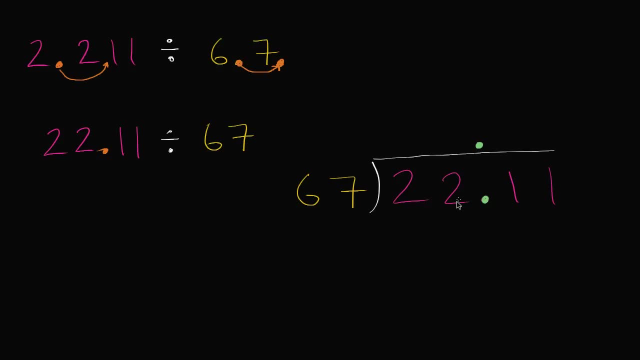 it's really important to write things neatly and keep things in nice columns and keep track of your place value, because if you don't write things in neat columns then, frankly, you'll probably lose track of your place value. So let's do this. 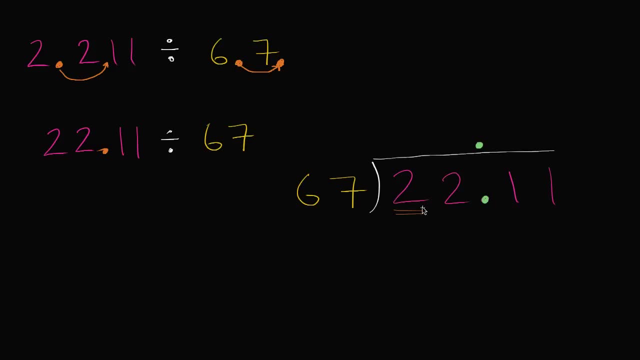 So 67 goes into two zero times. So let's move on. 67 goes into 22 zero times. 67 goes into 221.. So let's think about that a little bit. This is pretty close to 70.. 70 times three would be 210. 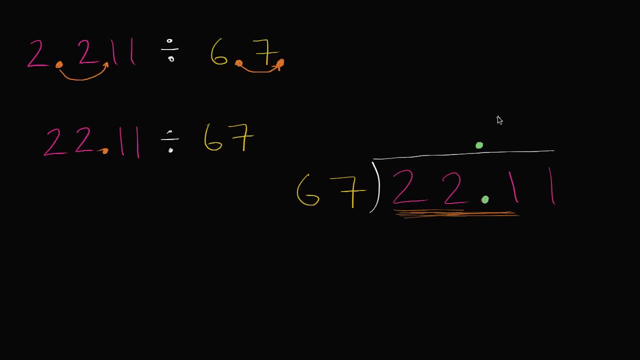 So this looks like maybe three times Three times seems about right. So let's try, let's put a three up here. Three times seven is 21.. Three times seven is 21.. Three times seven is 21.. Carry the two. 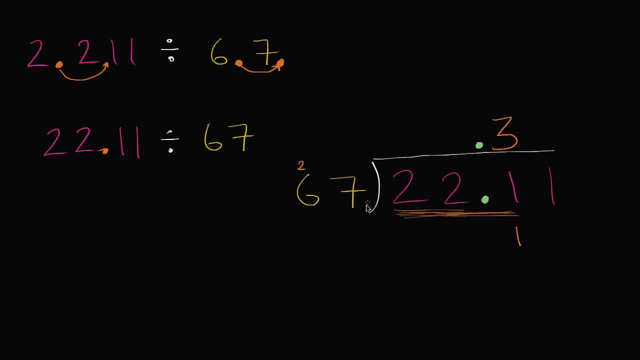 Three times six is 18.. Plus two is 20. Is 20.. So we get 201. And the difference between 221 and 201 is going to be: well, you just get a zero here. you get a two here. 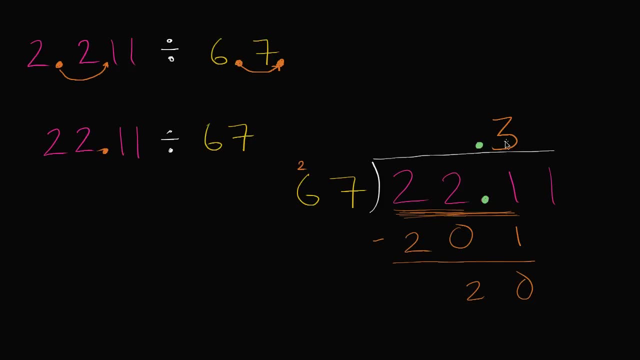 then you get a zero here. I don't have to write it, It's 20.. So three was right. If three times 67 were higher than 221, then we'd be in trouble. And then if three times 67 were lower. 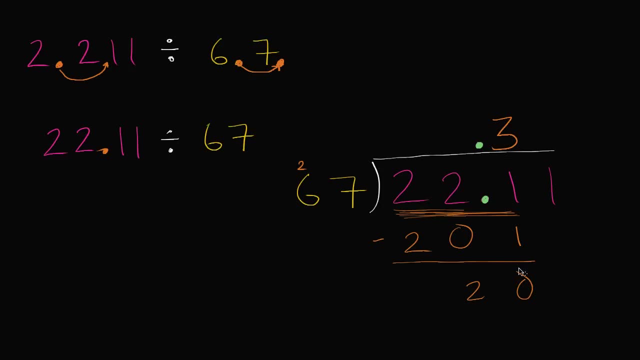 but it was so low that when you subtracted you got a number higher than 67, then that means you could have thrown in more 67s in there. But this number's just right. It's lower, but our remainder is less than 67.. 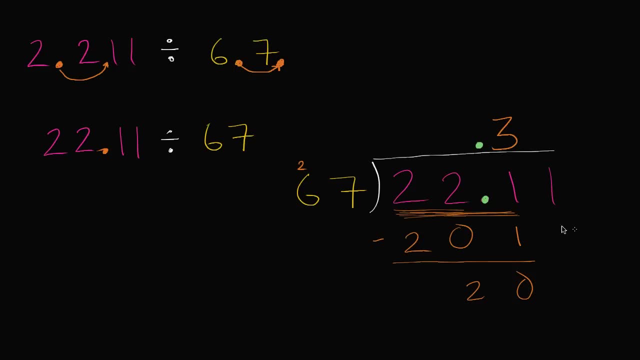 So let's keep going. So now we can bring down the one And we see 67 goes into 201.. Well, we just figured that out: 67 goes into 201 three times Three times Three times seven is one. 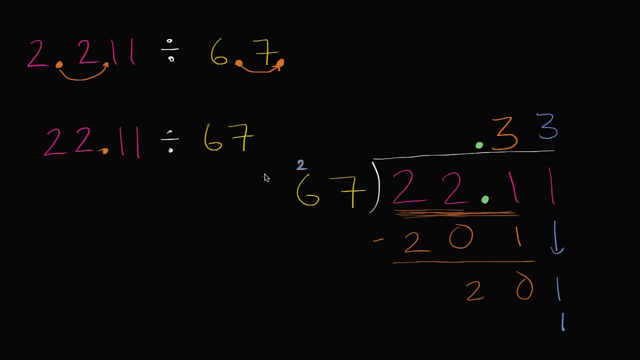 Carry the two. We've got to make sure we don't. well, we're doing the same problem as we did before, but it's good to not have the previous two there. Sometimes you might want to erase it And you have three times. six is 18,.